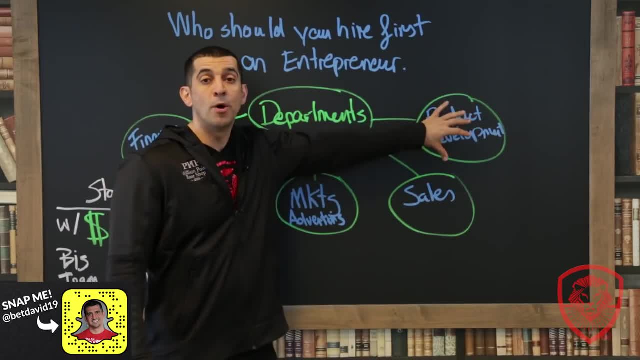 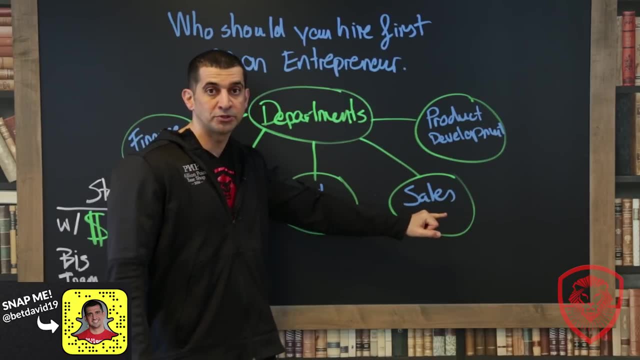 in sales If you're incredible at product development. most product development people don't like to be around a lot of people, So you need sales. If you're in sales and you're a great salesperson, like me, you're going to get inside the sales department, Whatever. 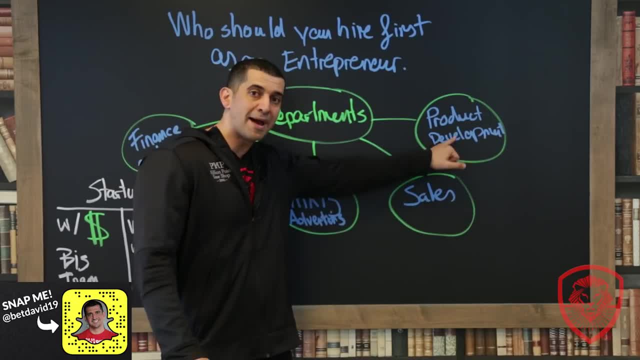 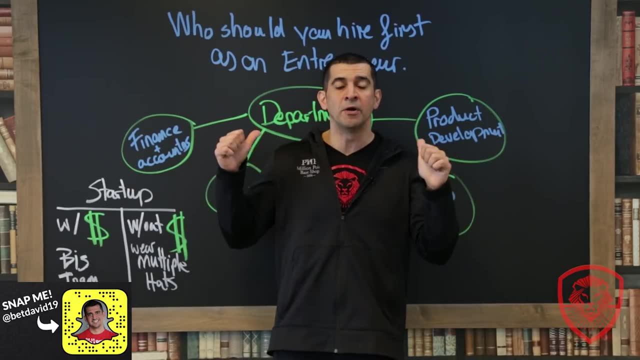 like Ray Kroc, but you don't know what product to develop. you need somebody here. If you're someone who's very good with money- and maybe even you have money but you don't have an idea- maybe you meet up there. 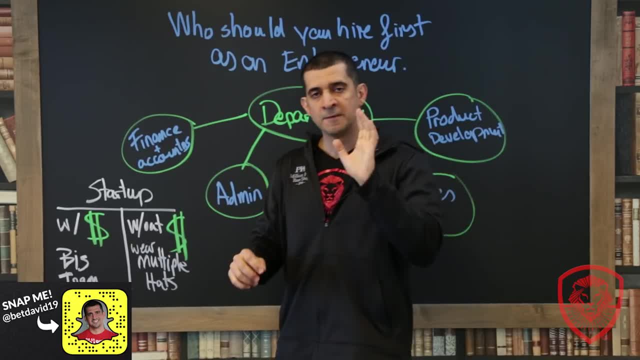 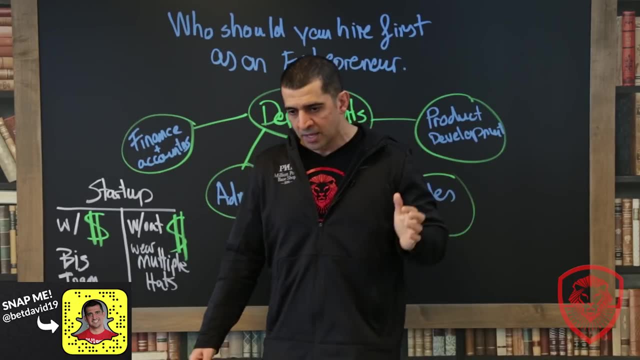 But the point I'm making to you here is: whatever your opposing strength is, that's what you need to start off with. Now let's say this other thing for you to be thinking about. I'll go dig a little bit deeper. In the game of sports, everybody that builds a team- they generally build it around their 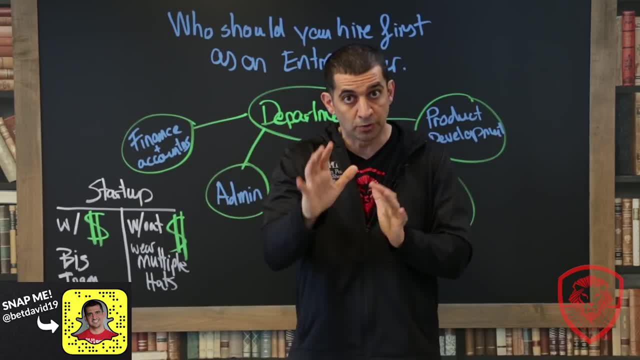 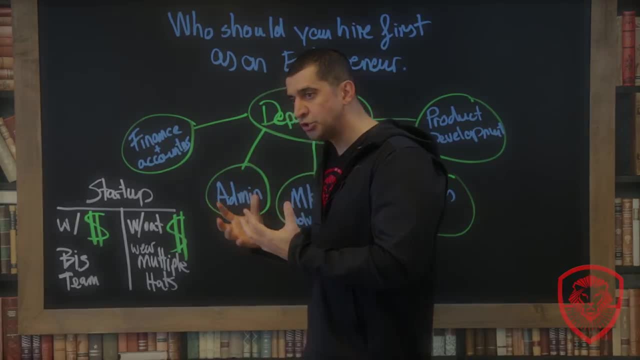 philosophy of what's the most important thing to invest their money into. Let me explain what I mean by this. Some teams build around one player. So, for instance, Chicago Bulls, Michael Jordan. they built around one player. Michael Jordan was the main player. 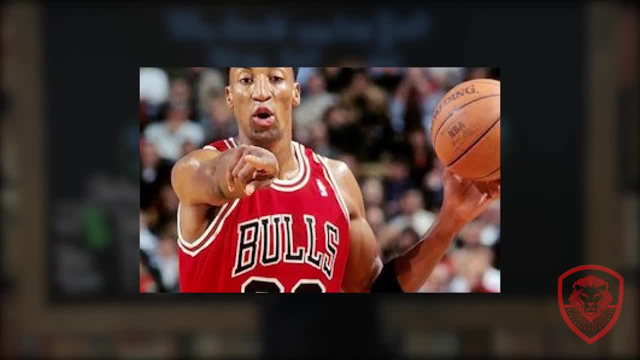 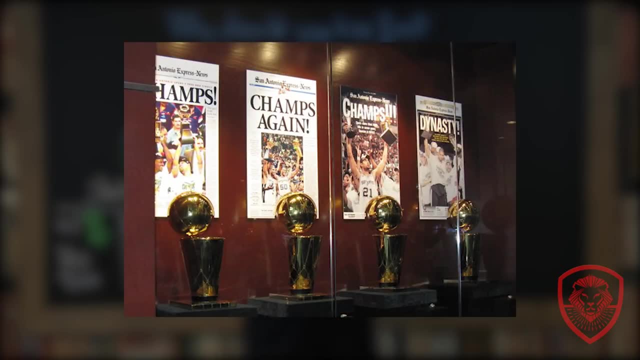 Then they brought supporting cast to be around them. San Antonio Spurs builds around a system. They're not building around one personality, one player. That's why they've been playing for 20 years and they're winning 20 years, Whether they go from. 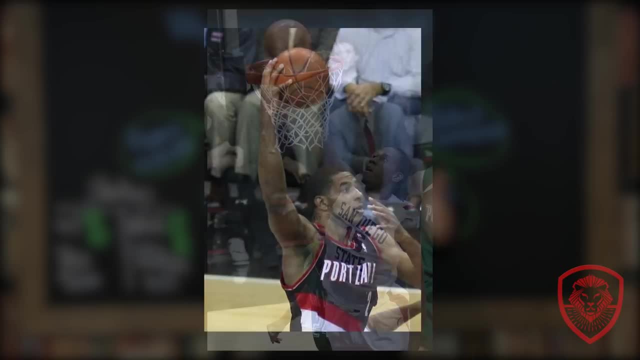 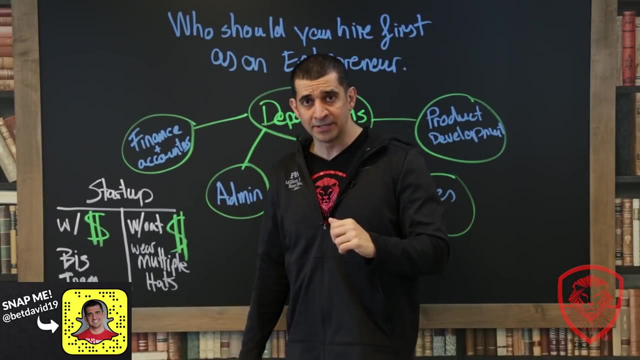 David Robinson to Duncan, to LaMarcus Aldridge and Kawhi Leonard. it's a system. they're building it on right. I don't know what you're going to be building your business and your philosophy and your system on, But what I could tell you is: whoever you choose as your first and next determines what you 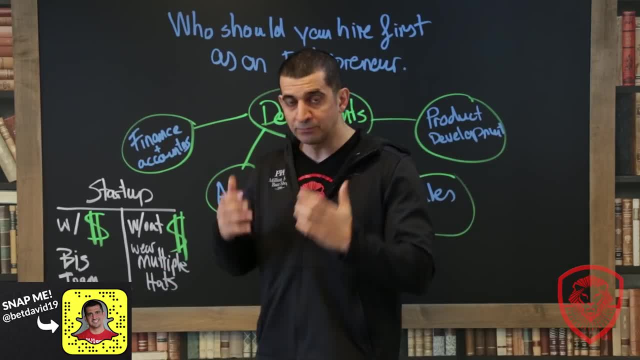 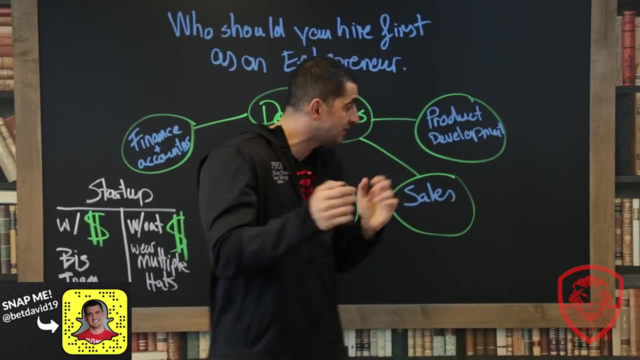 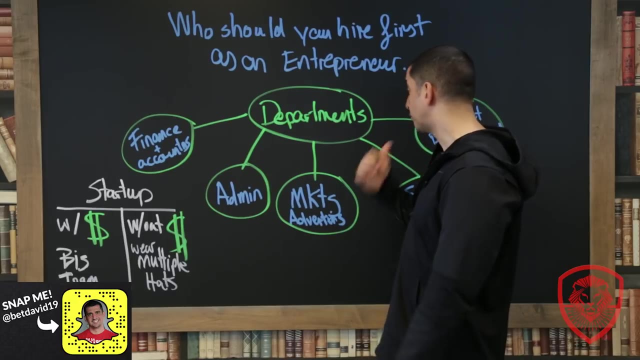 value the most, Sometimes generally the most logical people, the people that are most essence and everything to them is very logical and very organized, Like the administrative. The administrative folks. Sometimes they think they need this, Sometimes they think they need product development only. 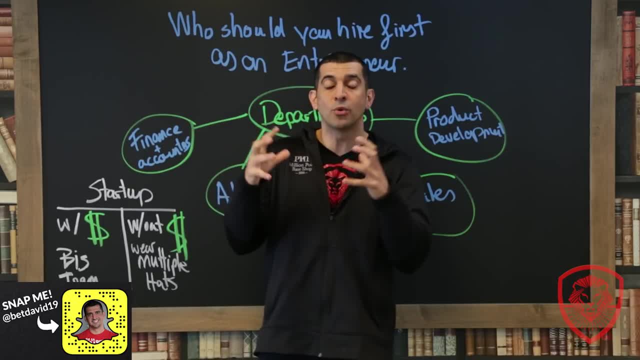 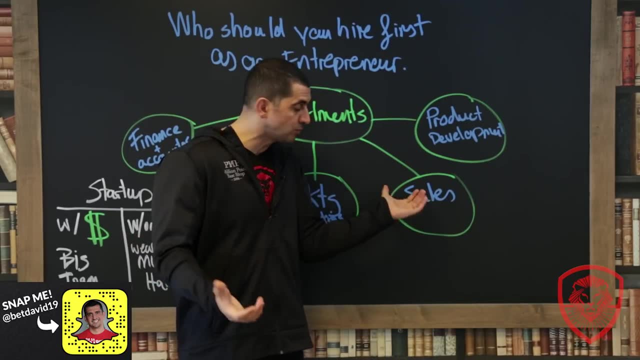 Logical. Sometimes they just go. everything is just way too logical and they forget that you need sales. If you don't have somebody selling, you don't have volume revenues coming in. If there's no sales going on, done, It's purely a done deal, right. 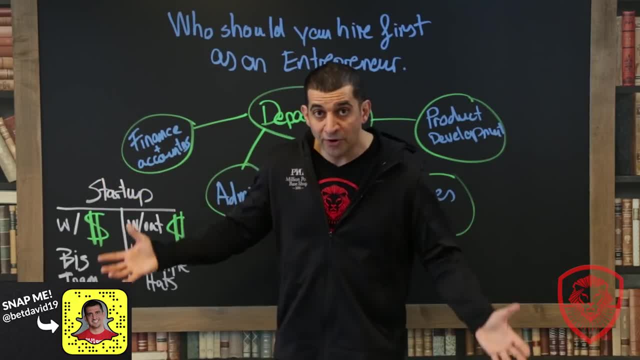 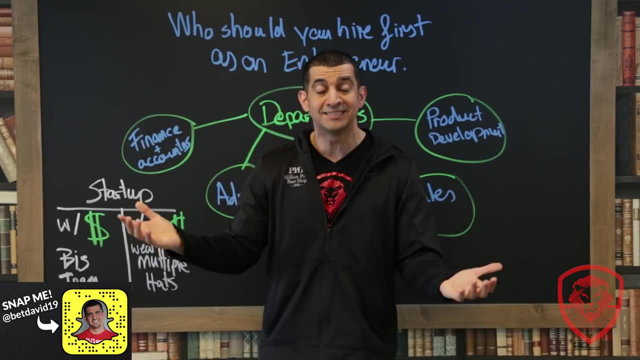 So back in the days when a lot of companies would do very, very well and they would develop these guys that would become the CEOs of the company, Everybody, Everybody that started with a company back in the 60s, 70s- you read about they all. 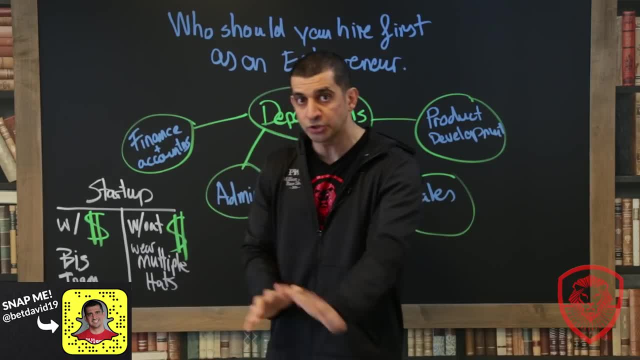 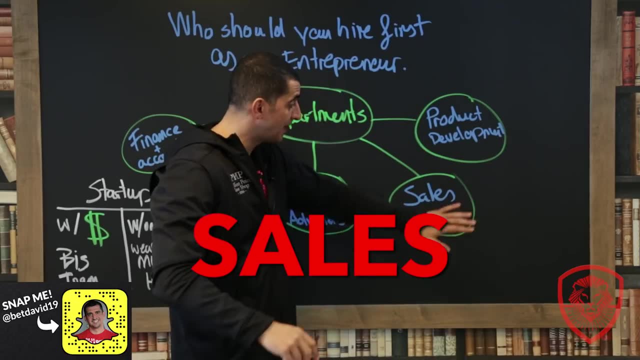 had to do sales at one point in their career. Why? Because they had to touch the customer to know what the customer is like. That is my focus. I like to hire this first. So if you're not sales, I like to hire this first. 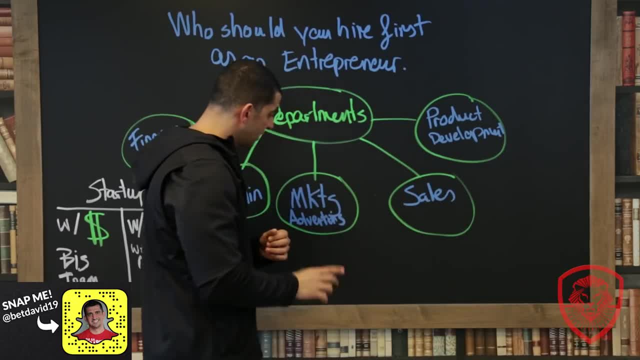 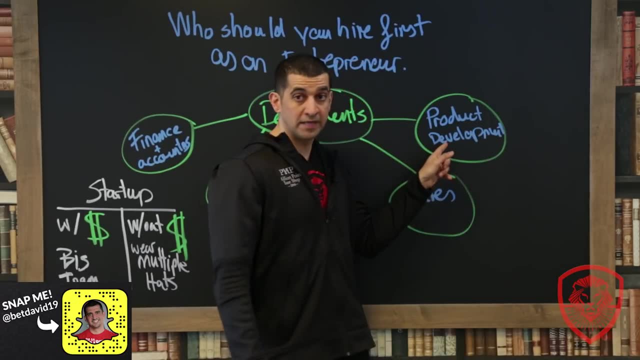 When I got started, I'll tell you for myself. I was this first and I'm marketing. This is me, So guess what I needed I needed here. I partnered up with here- somebody that designed the products that I needed. so without this, I don't have a product to sell. 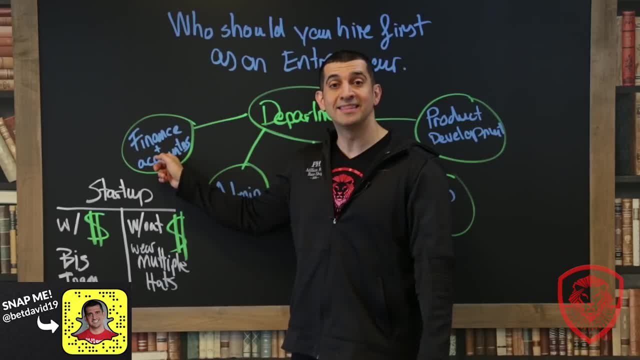 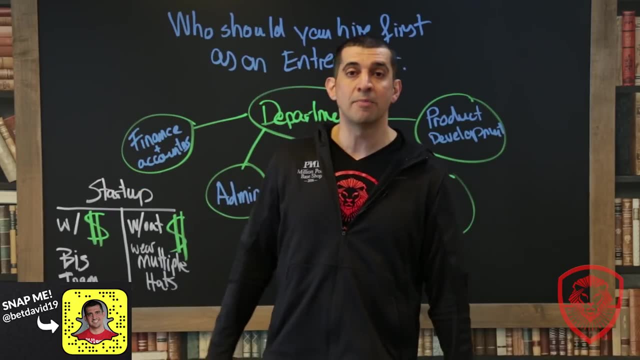 So I got product to sell and I needed admin. then I got this. I already had somebody that was helping me out with this, but then I got this. then I upgraded this to a whole different level. So, as you're thinking about this with your business- whatever business you're running- 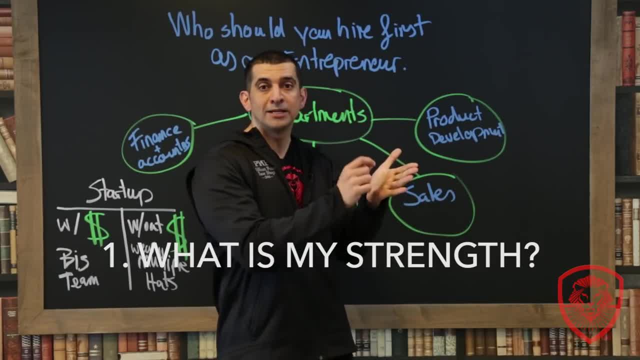 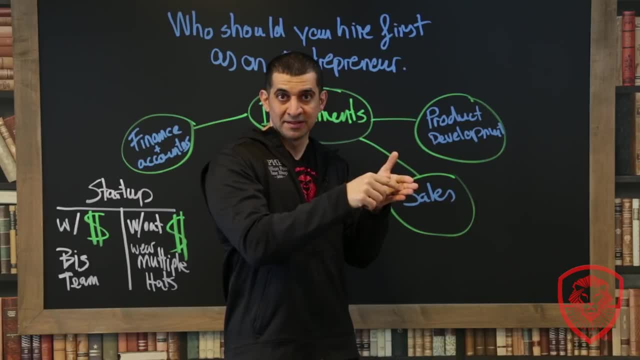 take this sheet of paper out and ask yourself: what is my strength and what are the opposing strengths that I need? Go recruit that person. Go hire that person. Stop hiring people that are just like yourself. It's cool to be right Be around people that are just like yourself. 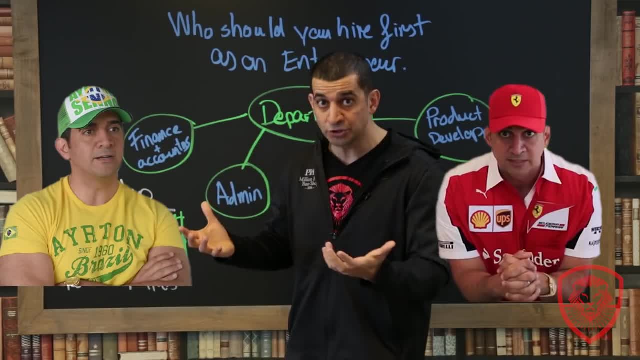 It's fun when you're around people like yourself. That's good, maybe when you have a friendship, but not when you're running a business. You're trying to create a business and a business. if you run out of this, you shut down the 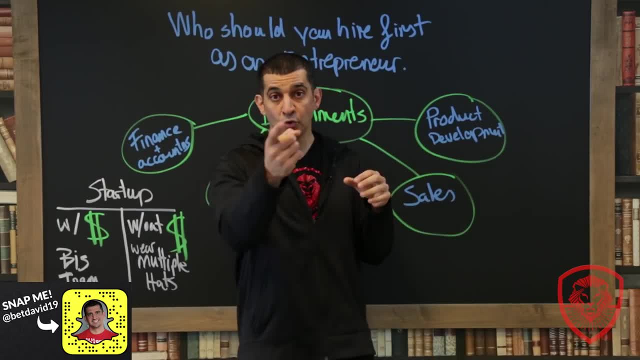 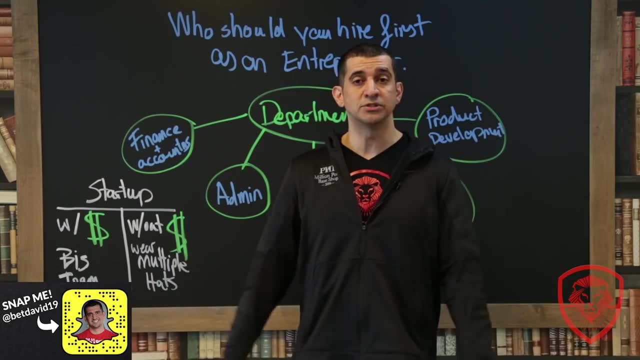 business. You're going back to having a job, So you've got to make sure you make the decision of who you hire first in a very, very proper way, or else you won't be in business for too long. Hey, thanks for watching this video. 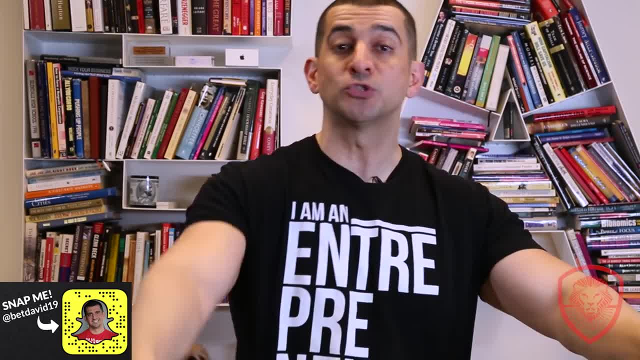 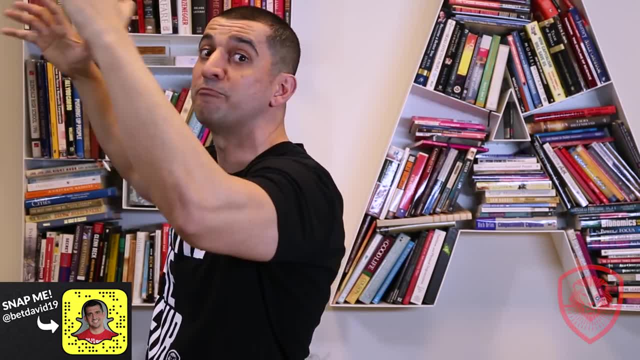 Let me make a case to why I believe you need to subscribe to Valuetainment and also join the notification squad. Look, there's two ways you can learn about business. One of the ways is go to college, Learn a bunch of theories by professors who have probably never ran a business before. 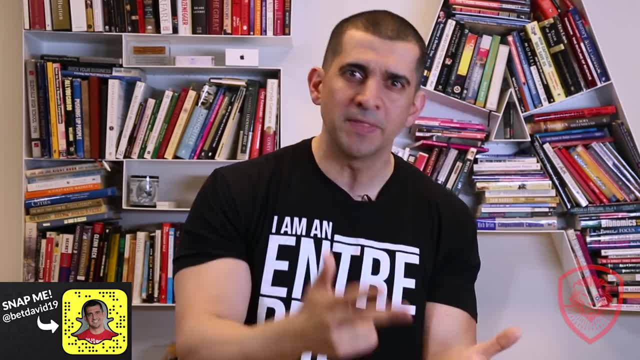 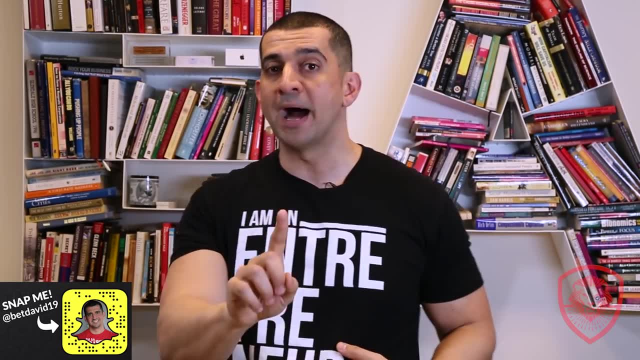 Or you can watch Valuetainment ran by entrepreneurs who have built and sold businesses, and you can learn from our mistakes and what we did right. And, by the way, I'm willing to bet anybody who goes and takes this boring route versus watches Valuetainment. I'm putting my money.